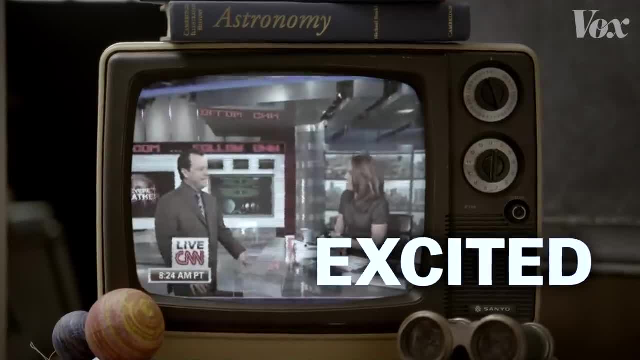 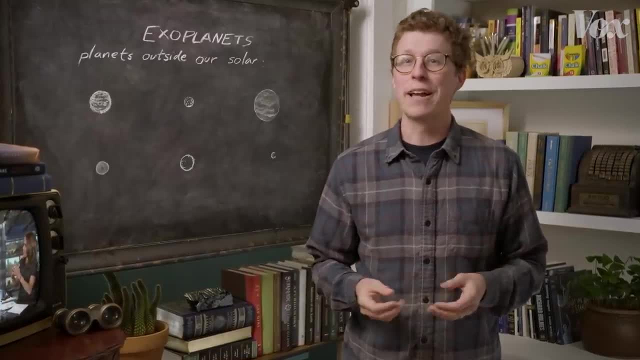 exciting. I am very excited. I'm excited. This is just really. this is so fascinating. I'm also excited, but I've always wondered how do people find these little exoplanets from trillions of miles away And how could they possibly figure out anything about them, their size, their 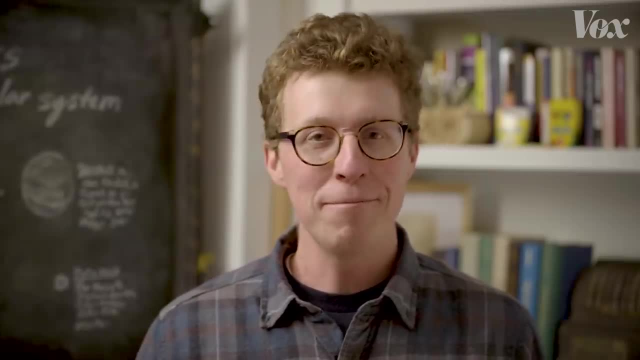 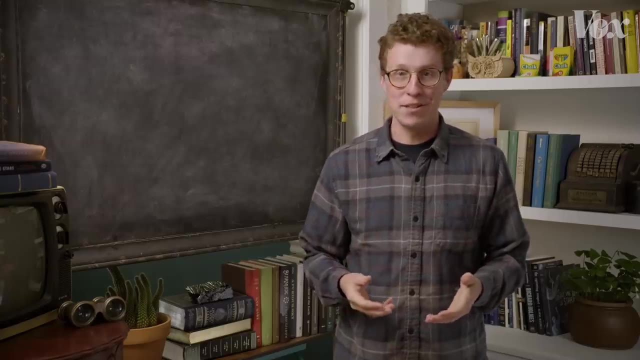 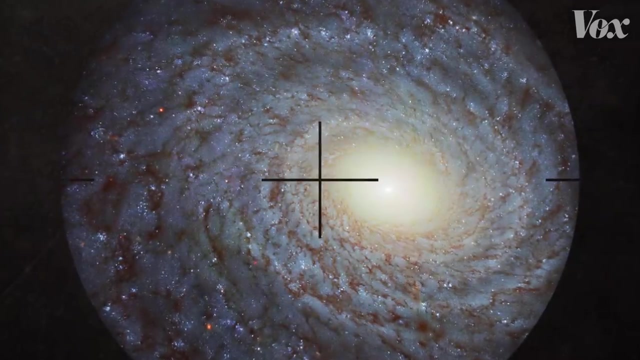 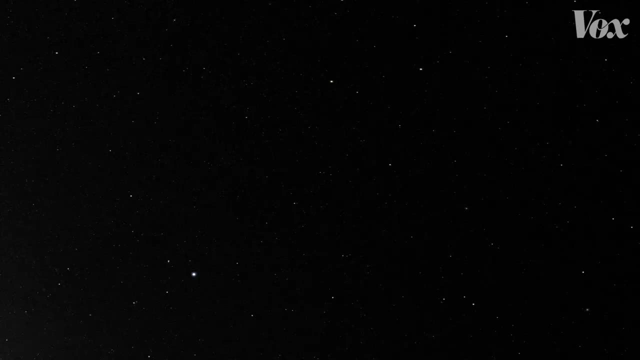 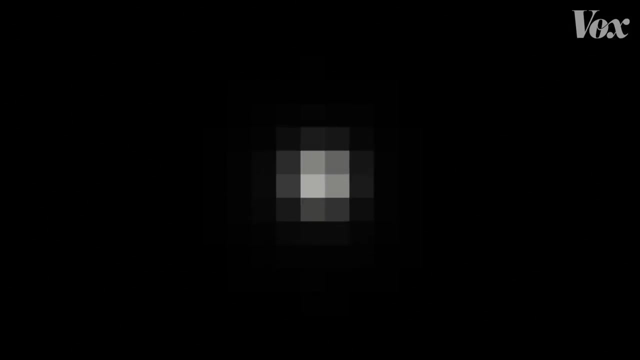 When we point our most powerful telescopes at stars that are similar to our sun, we get images like this: These pixels are capturing the glare of starlight, but the star is actually much smaller, and any planets would be smaller still, For example, if our sun were. 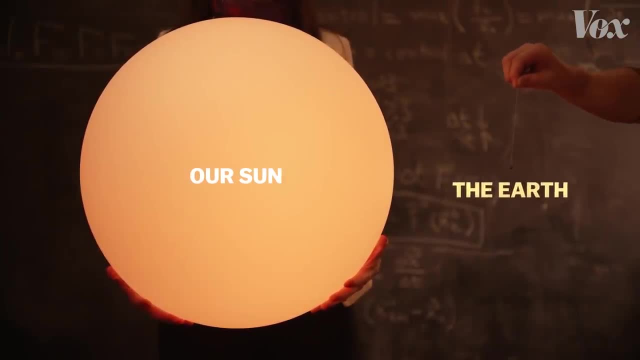 the size of this ball. the earth would be this big. If we're talking diameter, the earth is about a hundred times smaller than the sun, but the light reflecting off it is 10 billion times dimmer than the sun, So of course it would get lost in the glare. It's like looking for a 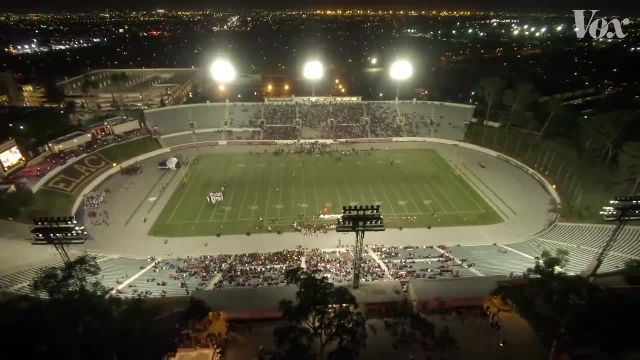 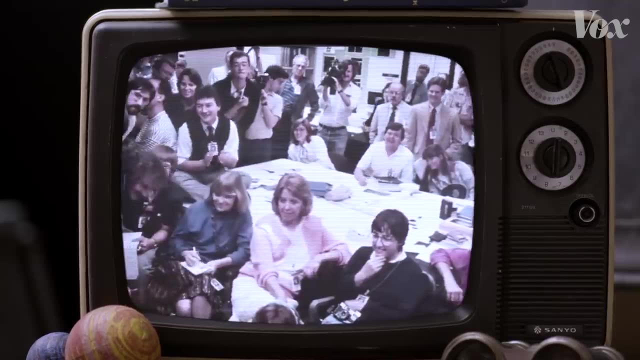 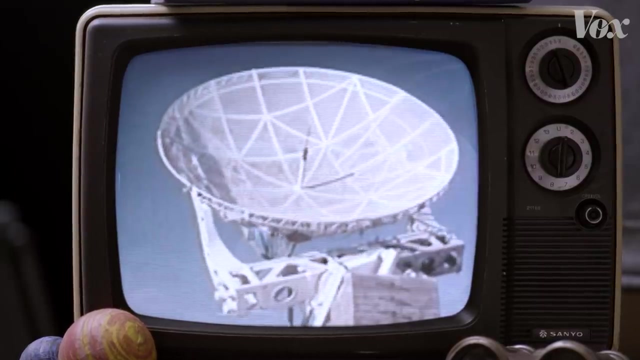 firefly next to stadium floodlights. In the 70s and 80s, astronomers set out to find a way around this problem. At that time, everyone was excited about finding intelligent life. We launched two interstellar probes that carried messages for aliens. Giant radar dishes started listening. 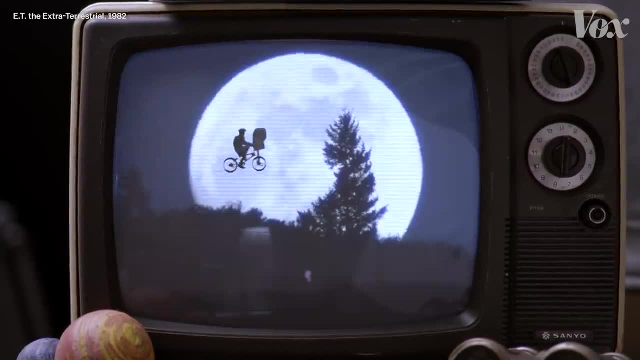 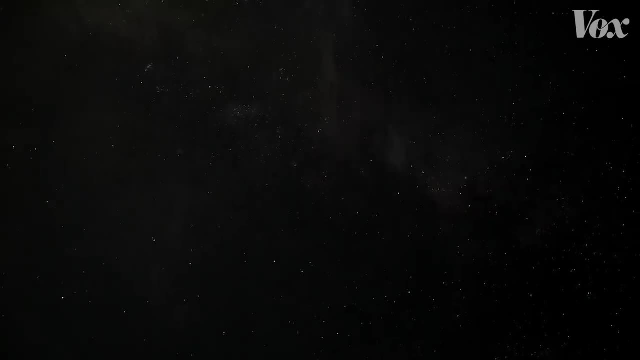 for voices from outer space, And ET became the highest grossing movie of all time. But in bare seemly, scientists had yet to find a single planet around another star. They had a pretty clear wish list. First, just confirm the existence of a planet. 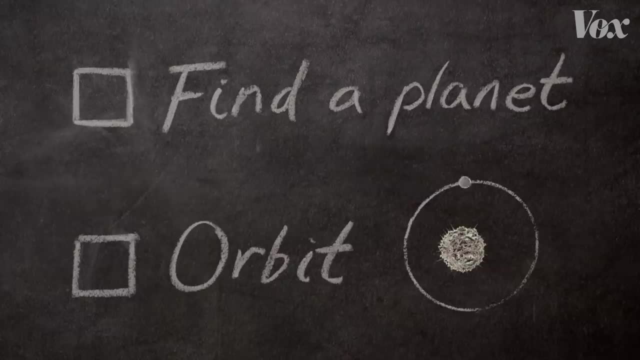 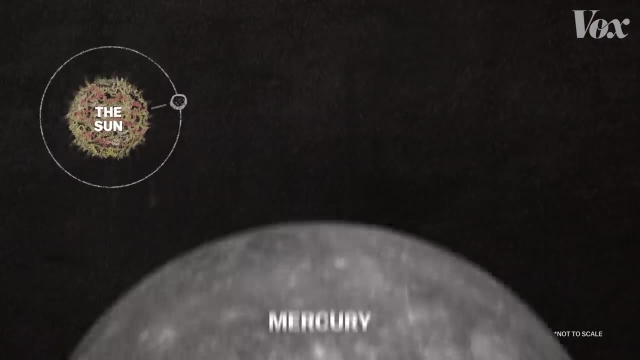 Second, find the size of its orbit. We'd really like to know the distance from the star so we can understand how warm the planet is. Is it a boiling hellscape? too close to its sun, like Mercury, Too distant, like Jupiter's frozen moon, Europa, Or just right? 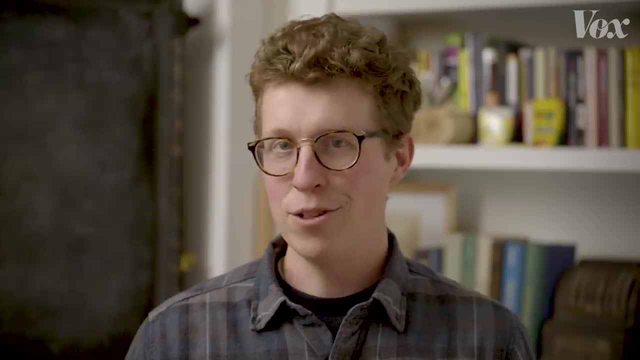 the kind of place that could have liquid water. Third, it would be nice to know the distance from the sun, like Mercury Or just right, the kind of place that could have liquid water. Third, it would be nice to know the distance from the sun, like Mercury Or just right. 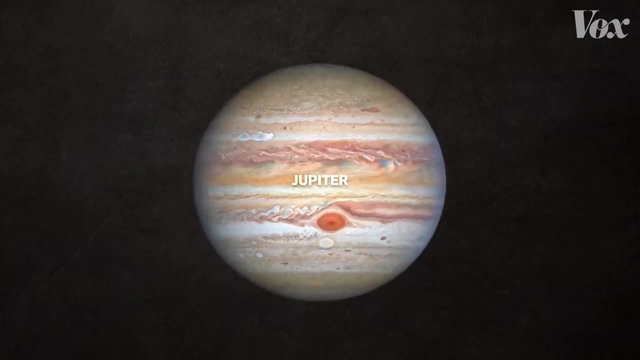 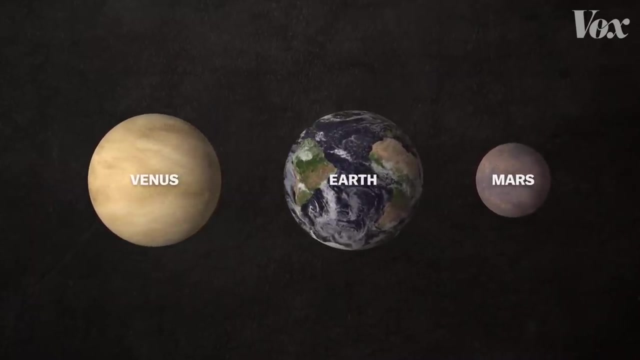 the kind of place that could have liquid water. Third, it would be nice to know how dense the planet is. Is it a giant planet like Jupiter, made mostly of hydrogen and helium, Or is it one of the prized rocky planets that's mostly heavier, more dense material And, most of all but hardest? to do? we'd like to find gases in the atmosphere that might be associated with life. Oxygen is a fantastic biosignature gas. Our atmosphere is full of it thanks to plants and photosynthetic bacteria. And if there were an intelligent alien civilization? 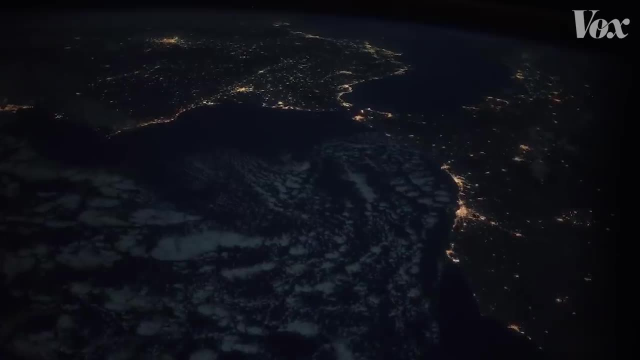 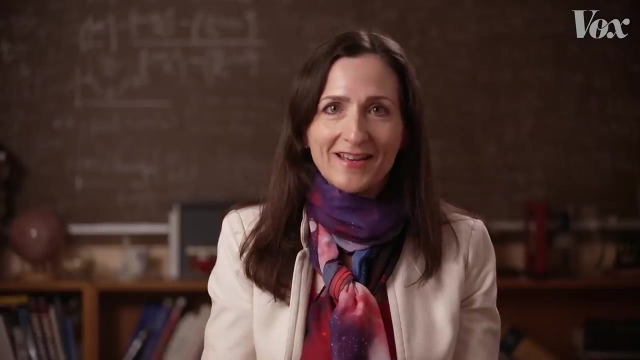 looking back at us, they'll be suspicious that something is here. It won't be our city lights or the Great Wall of China. It will be oxygen actually. So the goal was to find a planet, describe its orbit and its density. 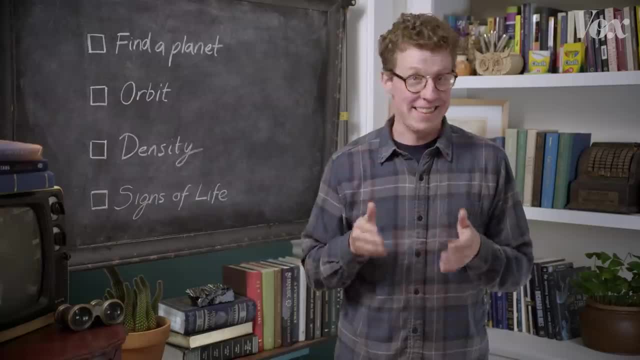 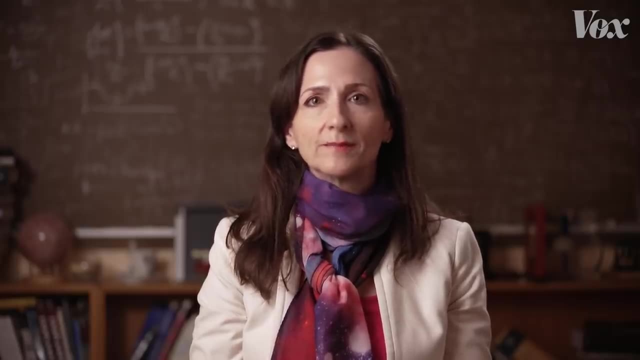 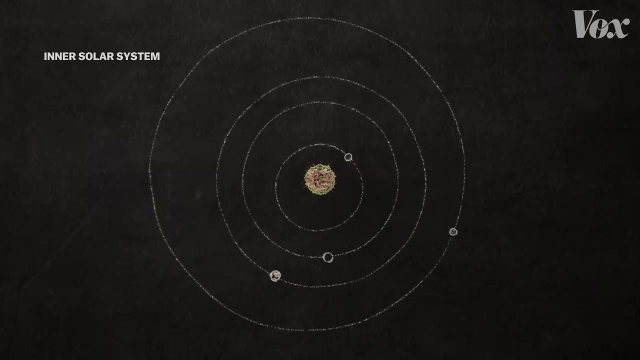 and search for signs of life, all just by looking at this. To detect or study an exoplanet, we have to work with the star. We sometimes think of our solar system, where our sun is a fixed point and that all the planets are orbiting the sun. 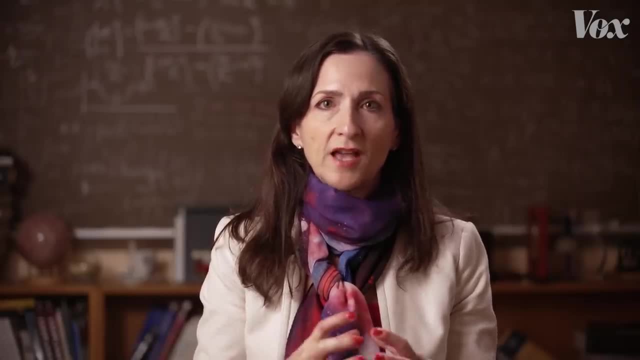 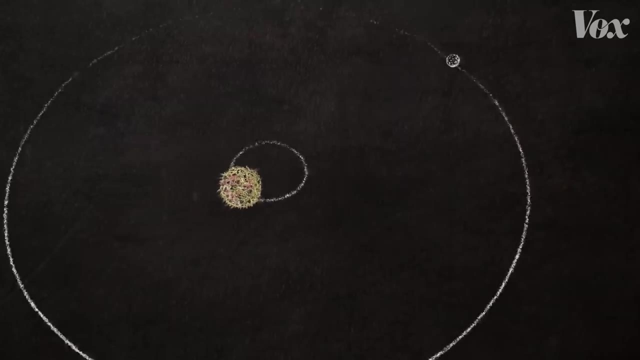 But a correction to the picture is our sun is not exactly fixed. The sun pulls on the planets but the planets pull back. The planets and sun are orbiting what we call their common center of mass And that makes the sun wobble back and forth. 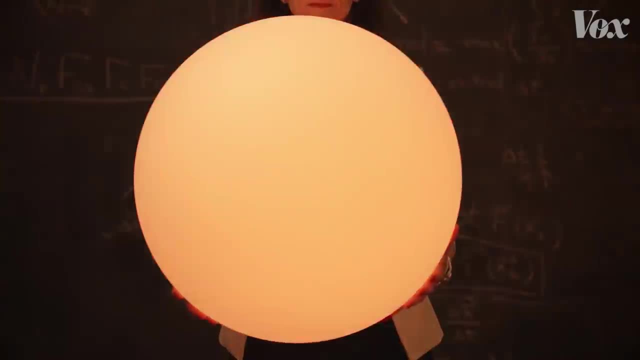 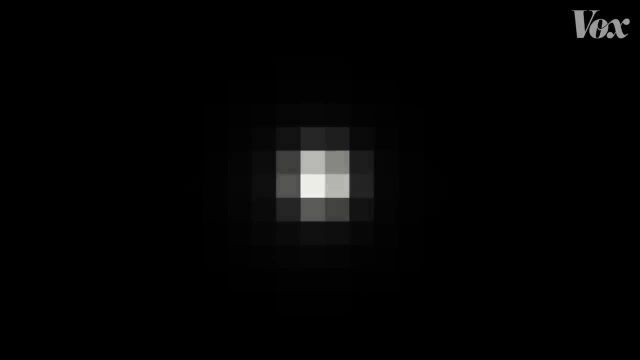 A huge planet will make the star wobble a lot, and a lower-mass planet will make the star wobble much less. We just had to wait for technology to get sensitive enough to pick up those wobbles. In 1995, Swiss astronomers announced that a star in the Pegasus constellation 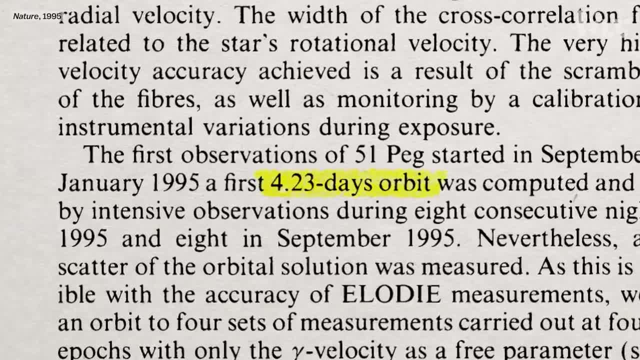 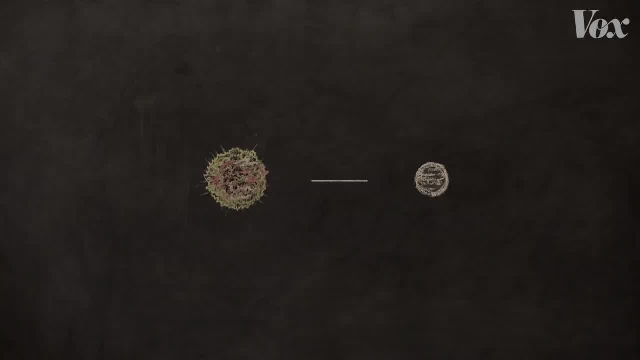 had an oscillation that repeated every 4.23 days. With just those data points, the basics of how gravity works and some simple math, They calculated that there was a planet only 4 million miles away from the star. That's incredibly close compared to our solar system. 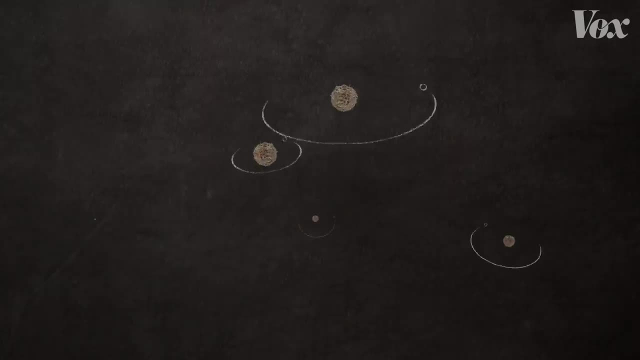 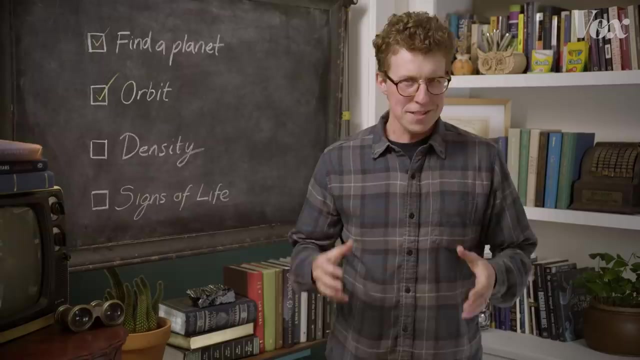 And it was about the size of Jupiter. Soon, the wobble method was turning up dozens of planets At the same time, revealing their distance from their stars, But this method couldn't deliver the precise mass or size measurements needed to calculate density. 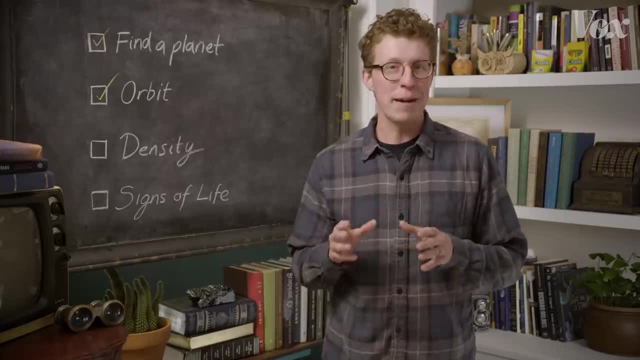 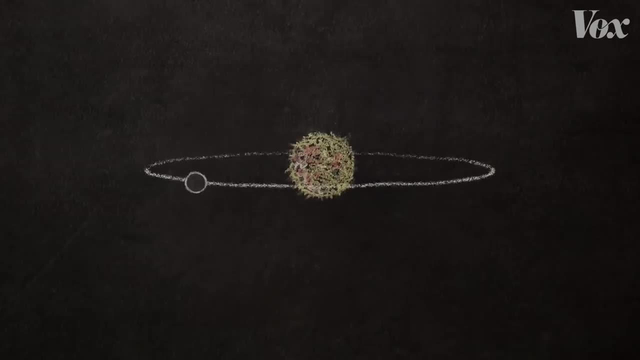 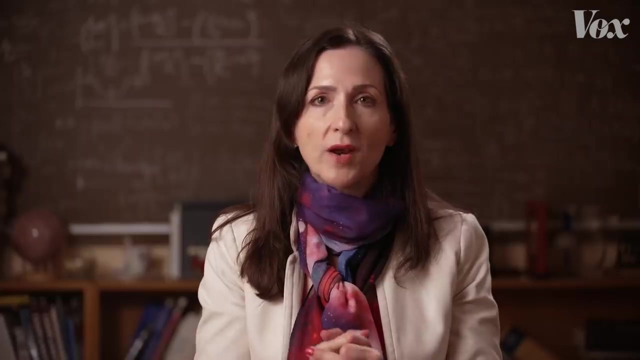 Luckily there's another way: we can indirectly detect planets just by staring at their stars. So some planetary systems are aligned just so, Such that the planet goes in front of the star as seen from our telescope, A so-called transit. And that's fantastic because we can monitor the brightness of the star and look for a tiny. 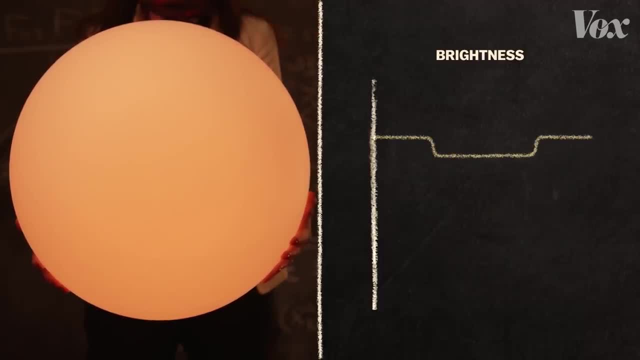 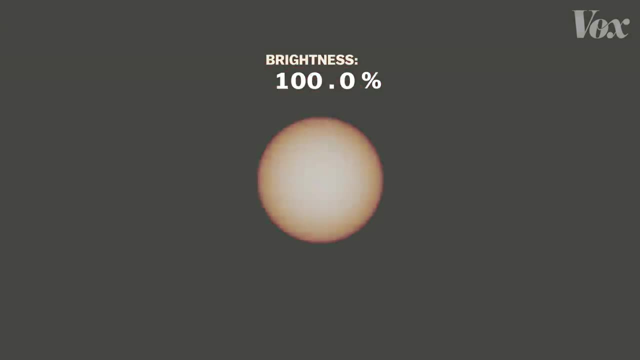 tiny drop in brightness That might mean a planet is going in front of the star. Our Jupiter's transit signal on our sun is 1%. Here's what that 1% drop would look like in our view of a distant star: Pretty hard to see. 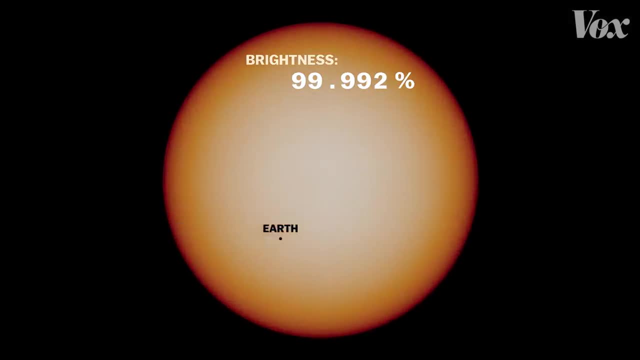 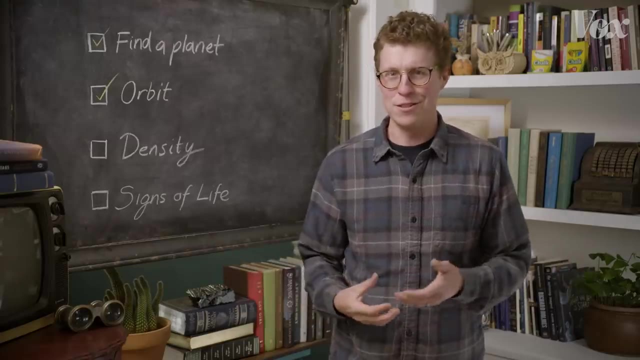 So for our earth and sun it's about one part in 10,000.. In the 1980s, no one knew how to detect a change that small, And most astronomers concluded that this so-called transit method was not practical as a primary. 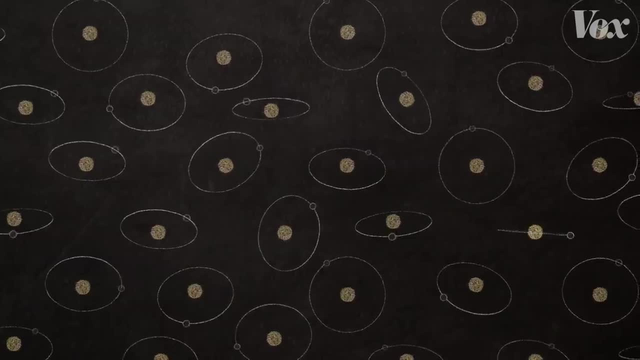 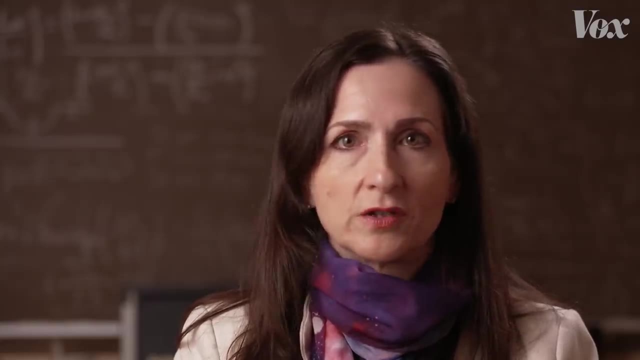 detection technique. It's very rare for a planetary system to be so perfectly aligned that we can see the transit, So we must monitor lots of stars, Tens of thousands or even hundreds of thousands of stars at a single time, And of course just seeing one drop in brightness isn't enough. You have to wait around for a second transit to know how long the orbit takes. If you were looking for Earth, that means you'd have to wait for at least a full year. It's hard. It's hard to find long period planets with the transit method. 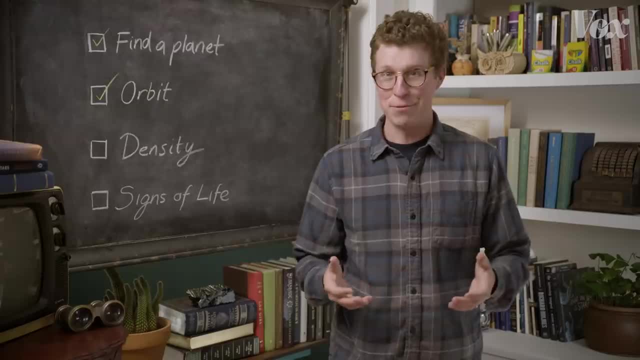 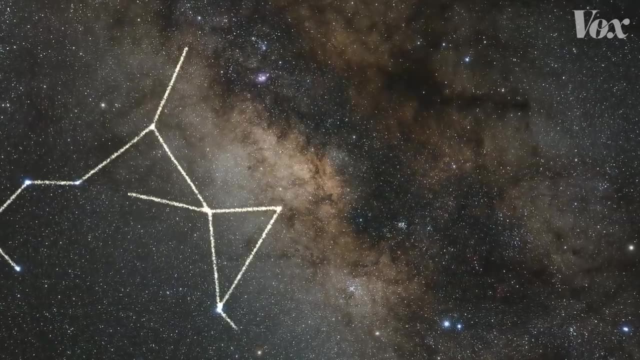 Because you have to be staring at one place for a very long time, But, as before, it was only a matter of time. In 2001,, a research team was watching five million stars in the neighborhood of Sagittarius, and they picked up a dip in the brightness of this one. 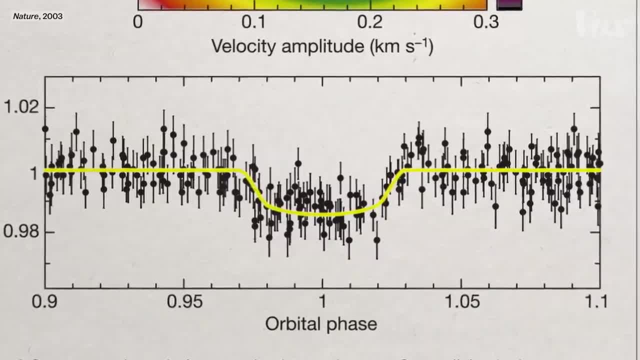 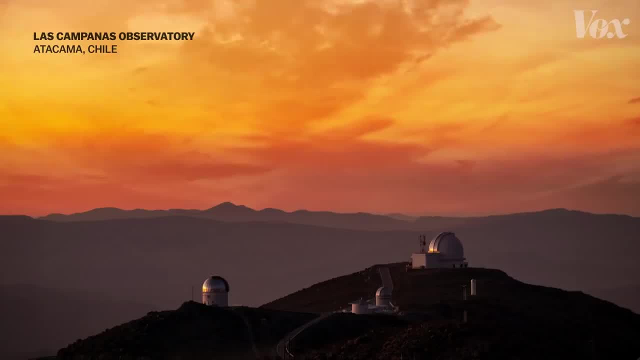 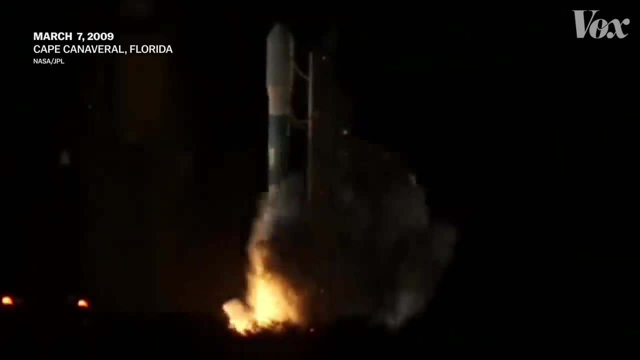 Luckily, they didn't have to wait around long for a second transit, because the planet they found shot around its star every 29 hours. The telescope they used was on the ground, which meant it had to peer through Earth's turbulent atmosphere. Not exactly ideal, but the Kepler Space Telescope, launched in 2009, was literally above all that. 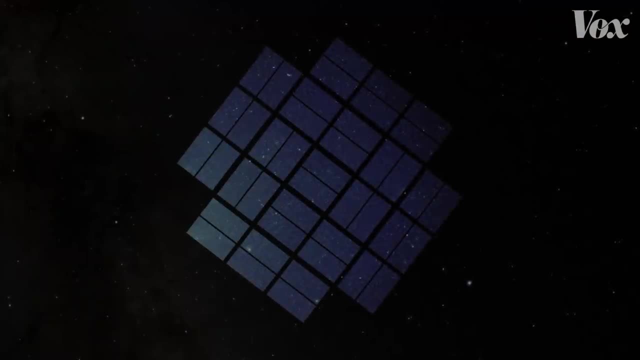 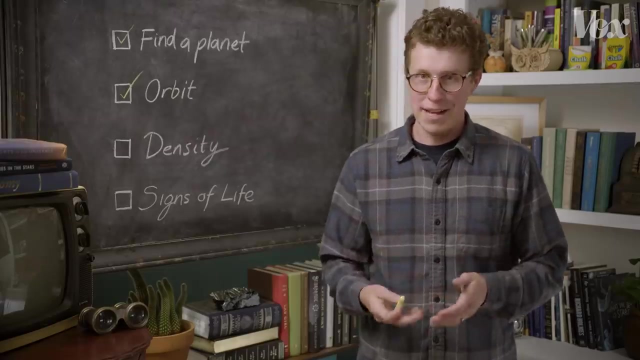 It watched one patch of sky for years and found thousands of planets. Not only was this a good detection technique, it could also be used to figure out the precise mass of the planet, and its size too. The bigger the planet, the bigger the drop in brightness. 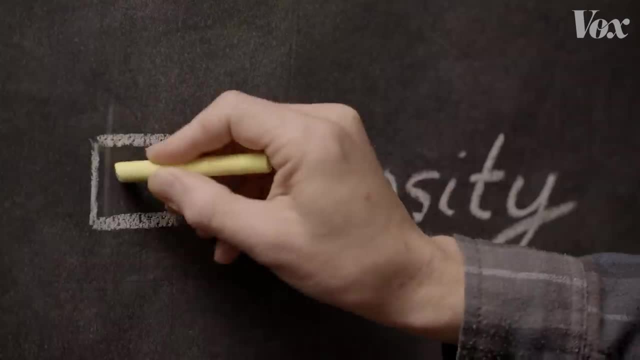 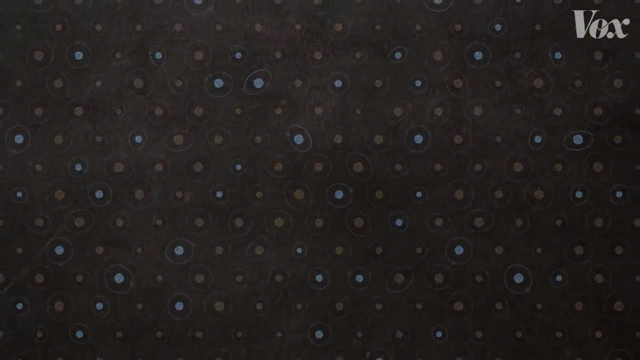 And with those elements you could finally calculate density. So far we've found nearly four million stars. There are over 5,000 planets, Hundreds are likely rocky worlds like Earth, and dozens of those seem to be in the habitable zones of their stars. 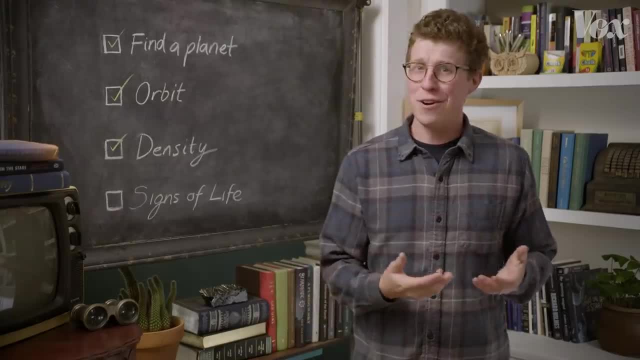 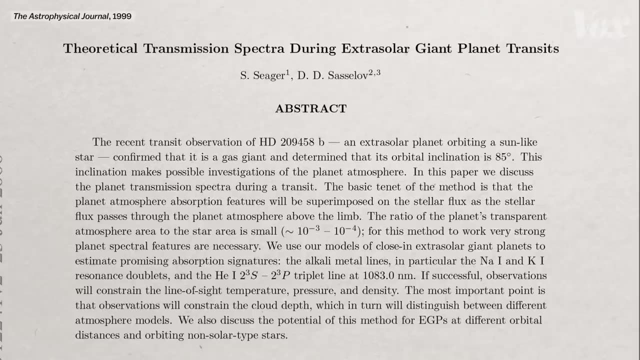 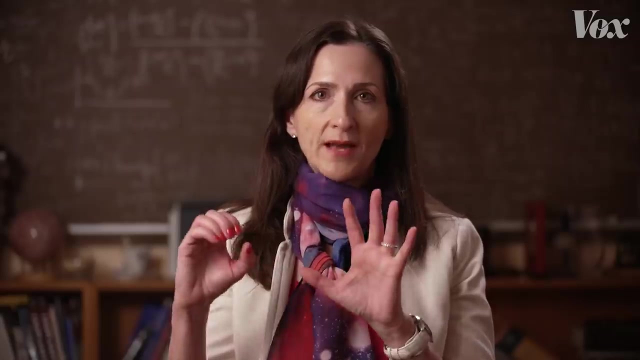 Incredibly, the question has shifted from do any stars have planets? to do any stars not have planets. But we're still looking for signs of life. How Well, back in 1999, Sarah proposed a way to investigate the gases in exoplanet atmospheres. 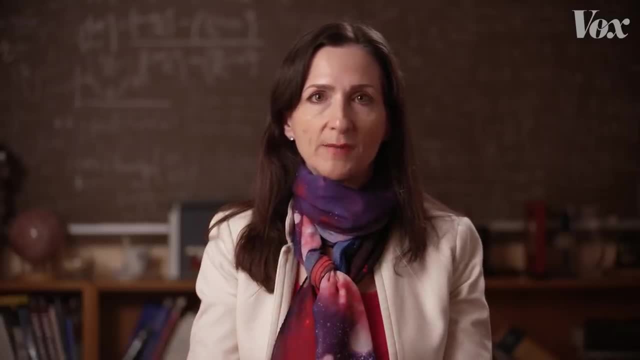 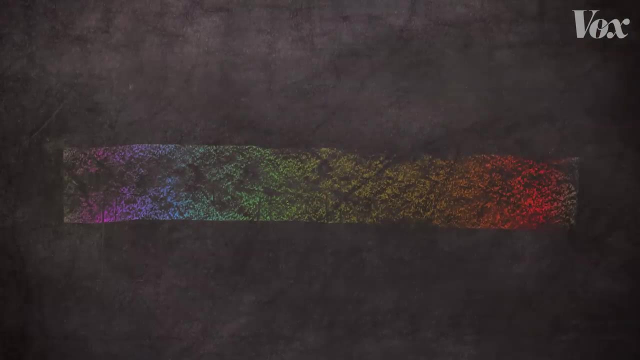 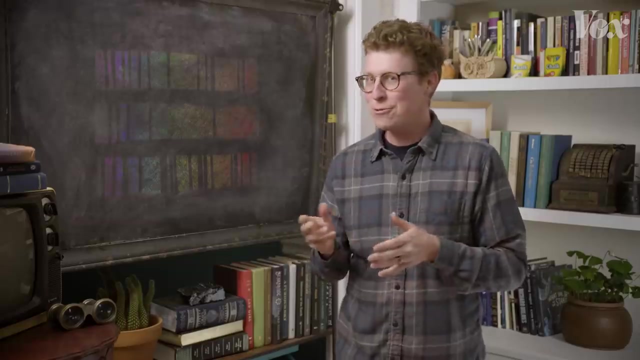 When that planet goes in front of the star, it shines through the atmosphere. Different gases in that atmosphere would absorb different wavelengths of light. For example, a simple molecule like hydrogen gas absorbs these bands. Other compounds have more complex signatures. Sarah's idea was to look for those tiny signals once that starlight reached Earth. 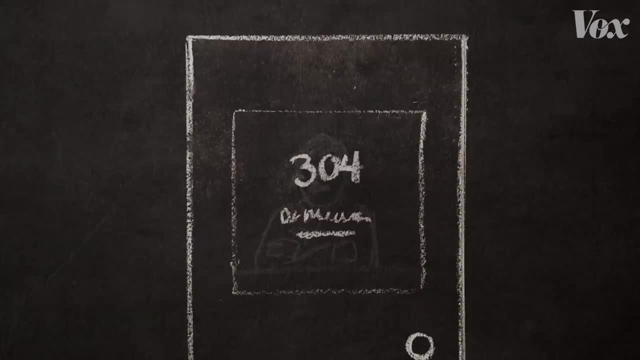 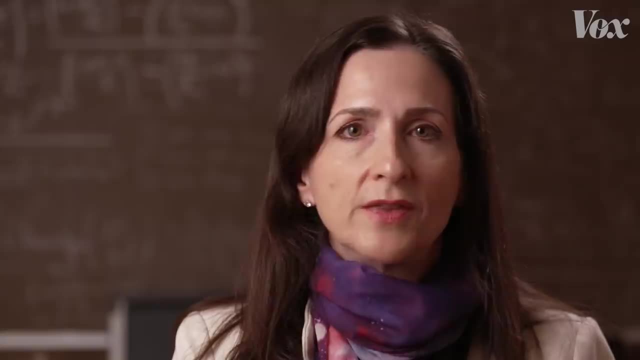 But not everybody was on board. So one place I applied for a job, a professor sat across from me and literally said: I just, I just don't think we're going to have very many transiting planets. They didn't think we'd be able to do that. 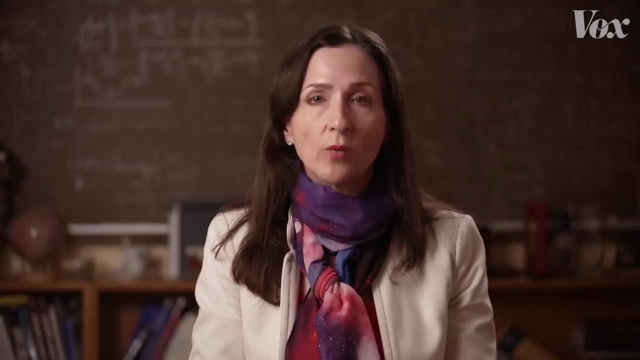 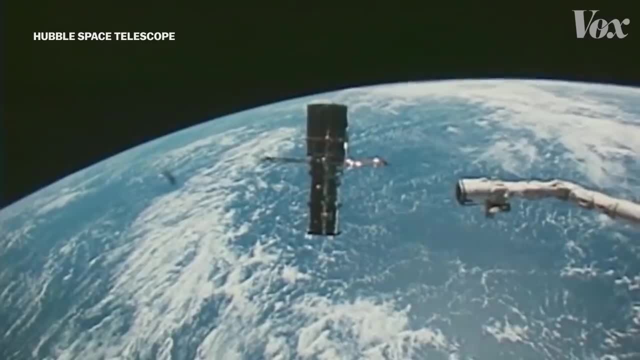 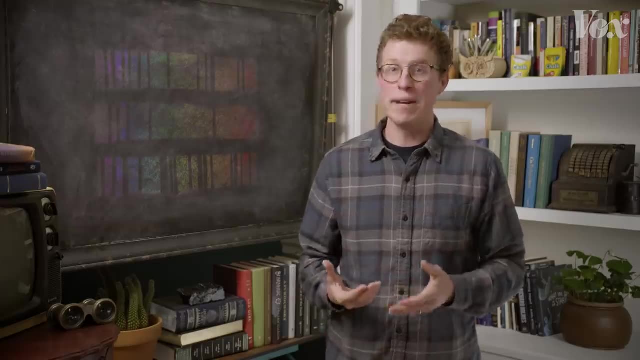 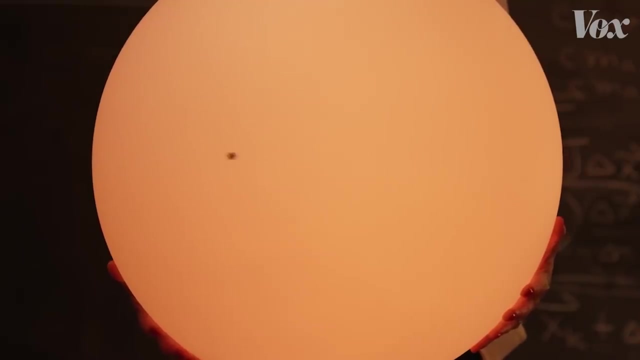 At least one team ran with the idea to use the Hubble Space Telescope and succeeded in observing the first exoplanet atmosphere. Unfortunately, it looks like this technique works best when the star is small and the planet is big. Earth-sized planets transiting sun-like stars have such a tiny signal. 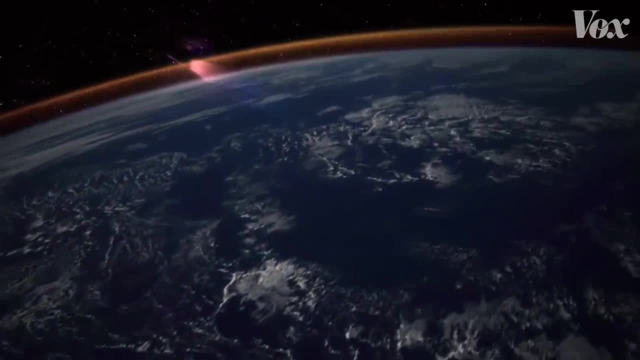 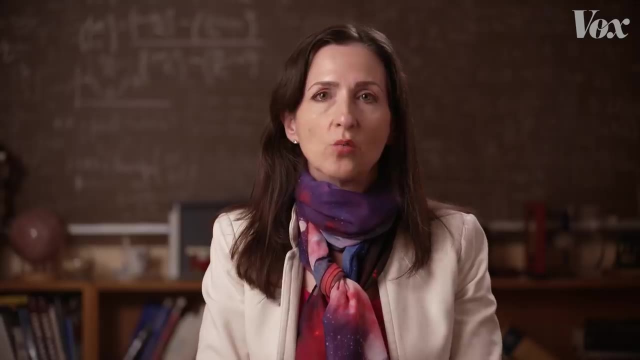 and their atmospheres have an even tinier signal that we may never be able to observe. It's like the skin of an onion on an onion. We need to move beyond transits to a different technique. We call this technique direct imaging. Okay, I know we started down this whole wobble and transit path. 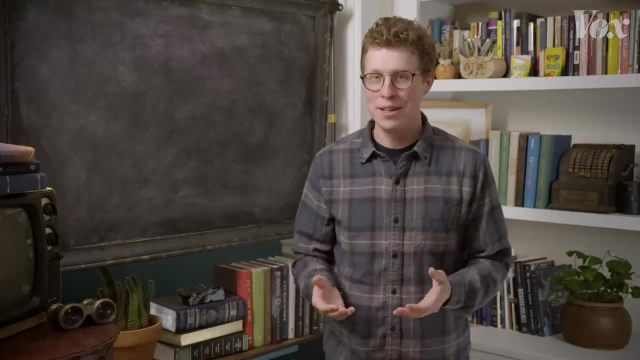 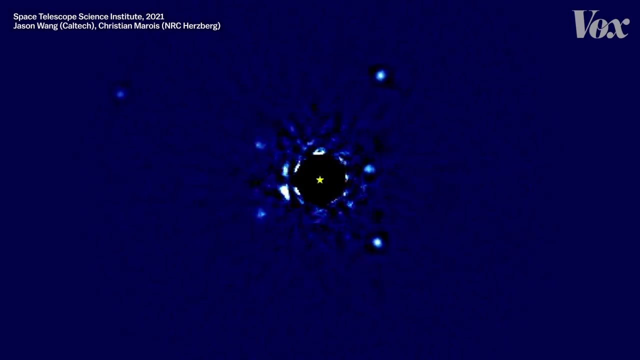 because taking a picture of an exoplanet seemed impossible. But look at this, This is a real time lapse of planets orbiting a star. The trick was to block out the star's overwhelming glare with a device called a coronagraph. Now this view is only possible because the planets are A really huge 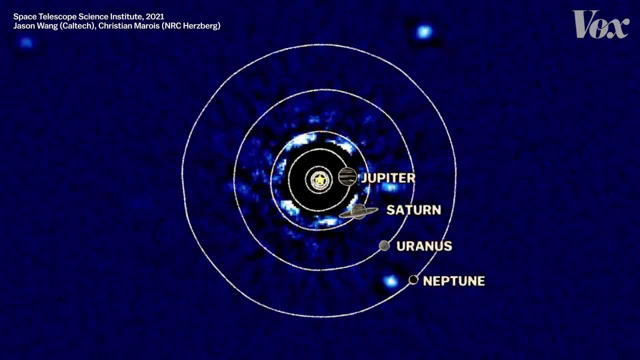 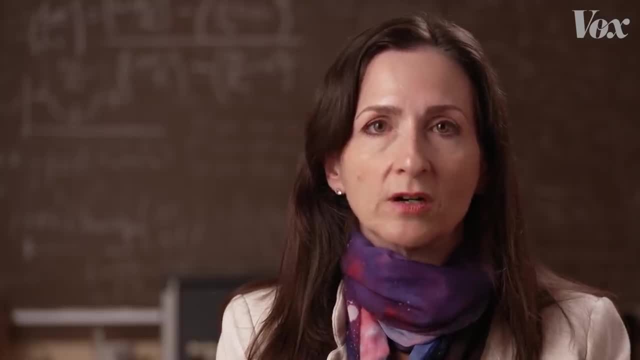 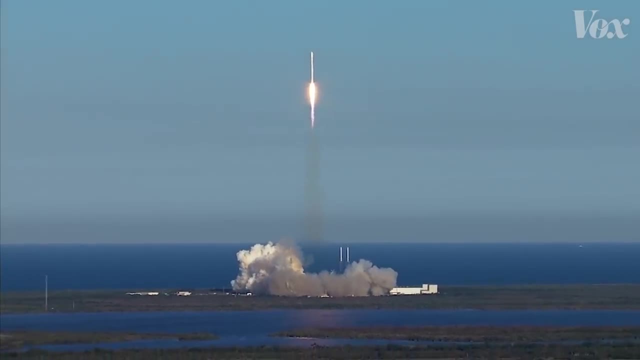 B, really far from their star. Here's our solar system for comparison, And see, they're all glowing red hot. We want to make direct imaging better and better so we can move down to smaller and smaller and cooler planets, And to do this we have to go to space to get.